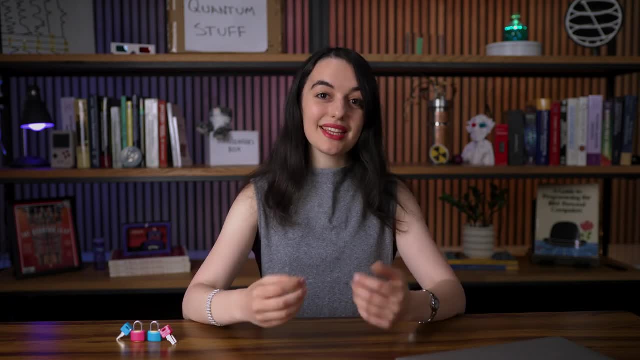 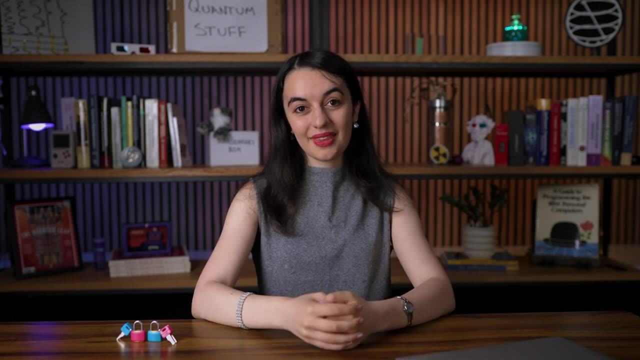 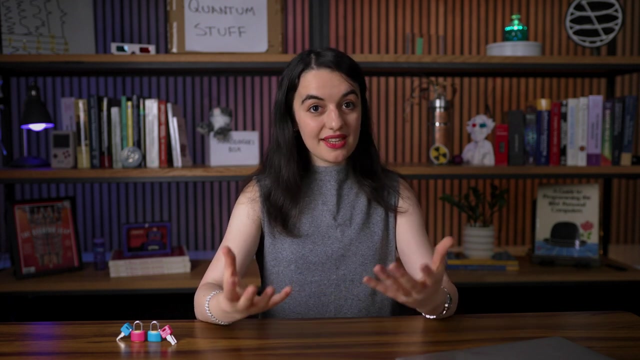 stronger constraint on the laws of physics, which requires that individual systems contain a complete mathematical description of the properties of those systems. Einstein's principle of locality is contradicted by many explanations of entanglement, which often say something along the lines of: if two systems are entangled, then measuring one system. 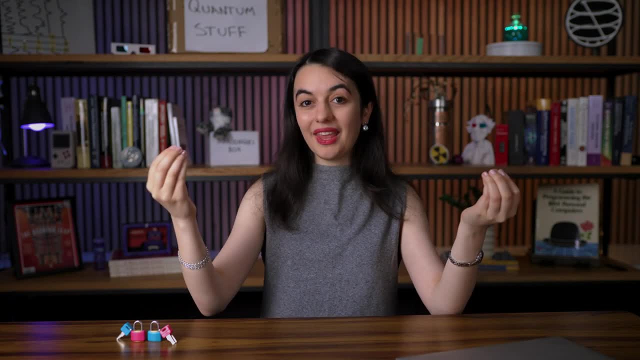 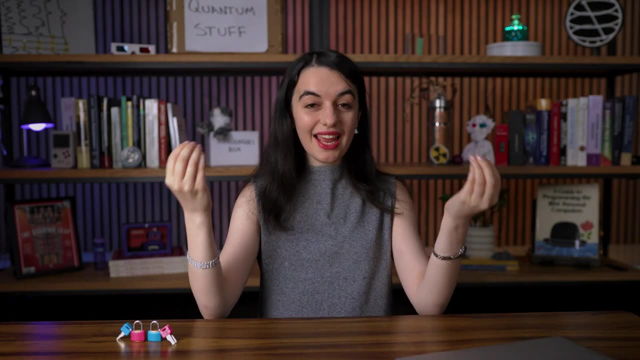 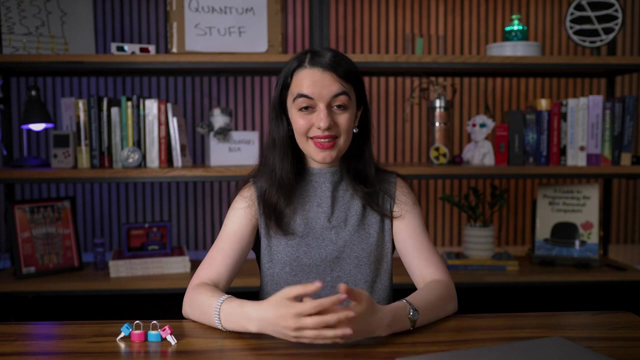 can instantaneously affect the other system, even if it's on the opposite side of the universe. Even with the caveat that this instantaneous connection cannot enable faster-than-light communication, it still violates Einstein's principle of locality. This kind of explanation of statement is typically backed up using bell's theorem, which was proposed by the scientist john. 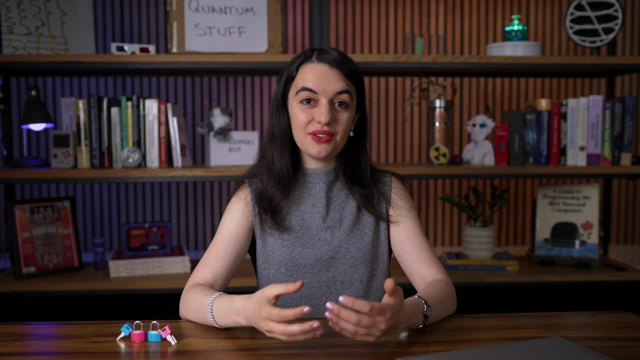 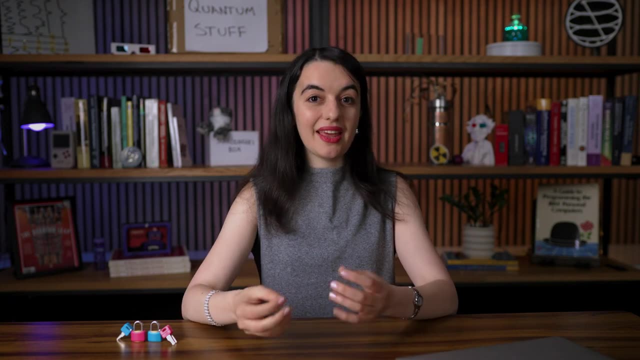 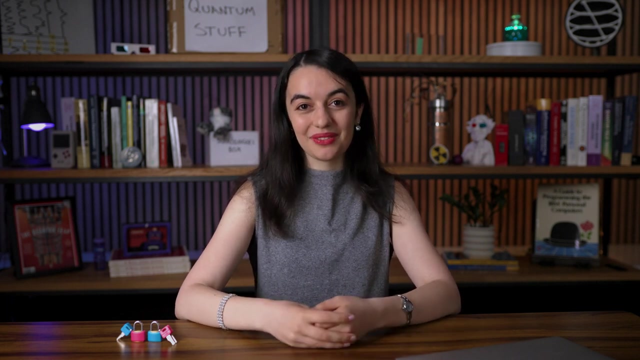 bell to show that the paradox can't be resolved by using a certain class of local theories, called local hidden variable theories. however, this doesn't mean that there has to be instantaneous effects between entangled qubits. we can, in fact, save einstein's principle of locality. 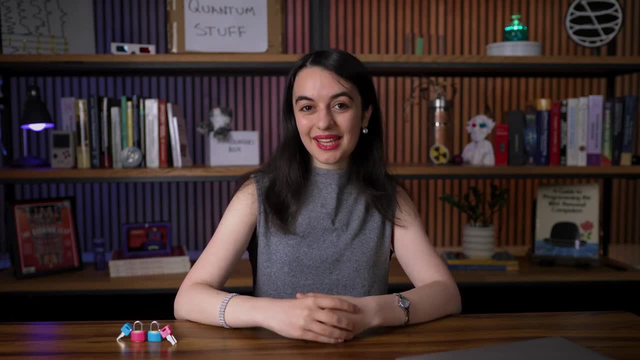 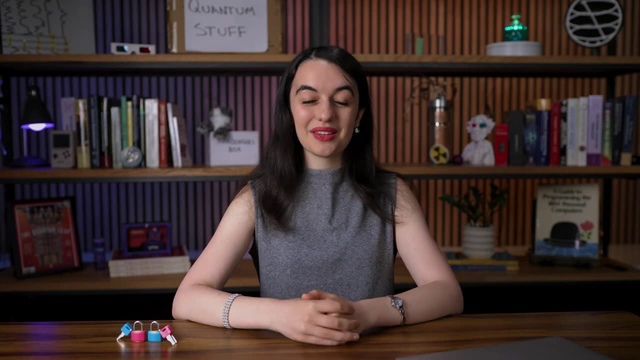 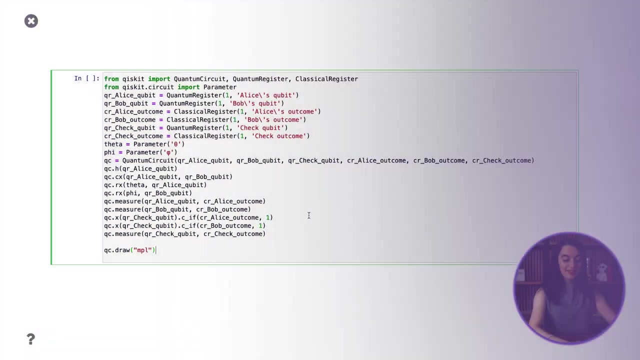 if you're not familiar with quantum gates and circuits, i recommend taking a look at the basics of quantum information course on the IBM quantum learning platform linked in the description, before continuing with this video. so now let's code this thought experiment using qiskit. here i've coded a quantum circuit for the standard EPL thought experiments setup. 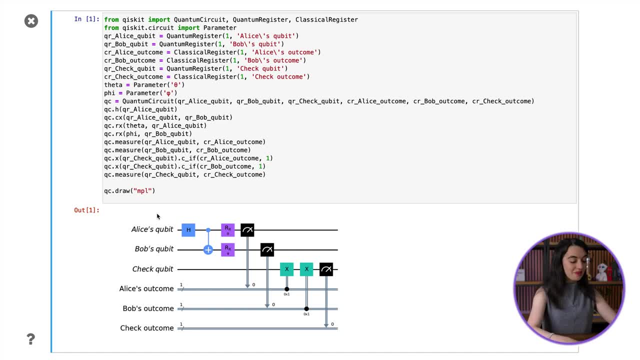 we have two observers, alice and bob. each have a qubit and their qubits are maximally entangled, which we prepare using a hadamard and a control knot gate to put them into a maximally entangled Bell state. Then Alice and Bob each choose a basis in which to 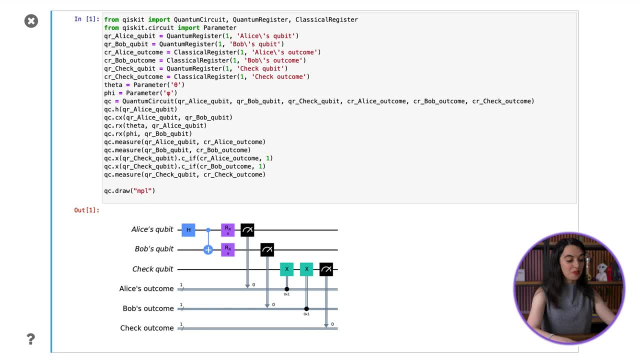 measure their qubit, which I've captured by adding a parameterized single qubit gate before each of them, doing a z measurement. For simplicity, I've made both of these gates be x-rotation gates, with Alice's characterized by the parameter theta and Bob's by phi, but in general they could both. 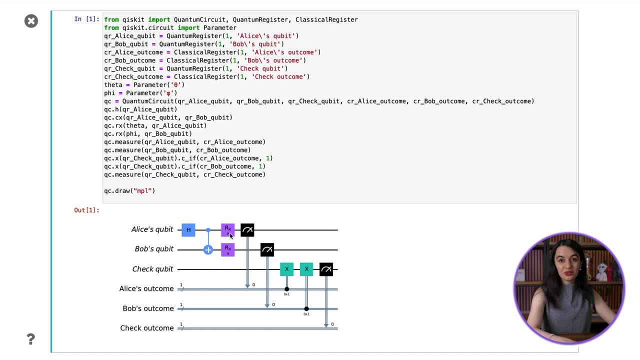 be a unitary gate u, where each u is defined by three parameters and the same explanation that I will give now will hold. Then I've introduced a check qubit which stores the outcome of a parity check on Alice and Bob's measurement outcomes implemented by a pair of control, not gates. 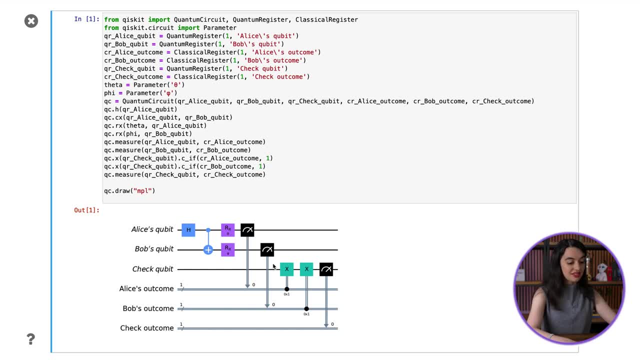 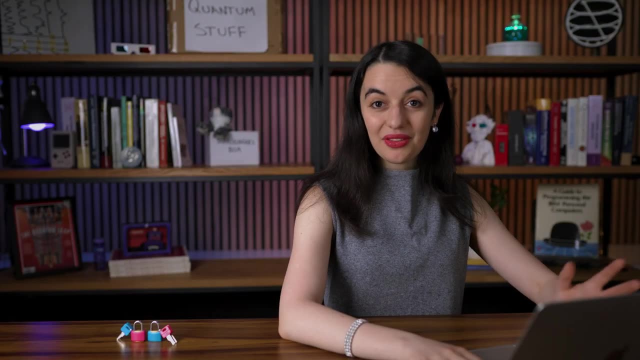 controlled on Alice and Bob's measurement outcomes and targeted on the check qubit, Then if Alice and Bob's measurement outcomes are the same, the check qubit will be in the zero state, and if Alice and Bob's outcomes are different, then the check qubit will change to the one state. Now the strange thing about measuring. 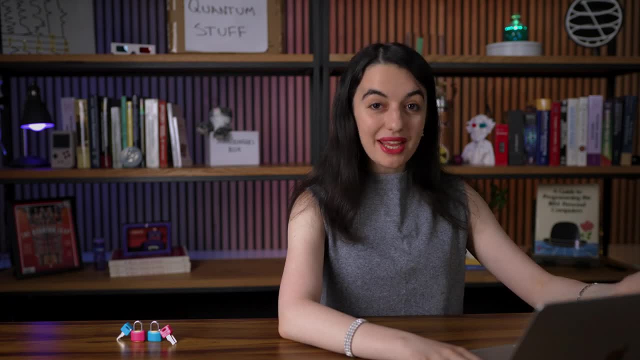 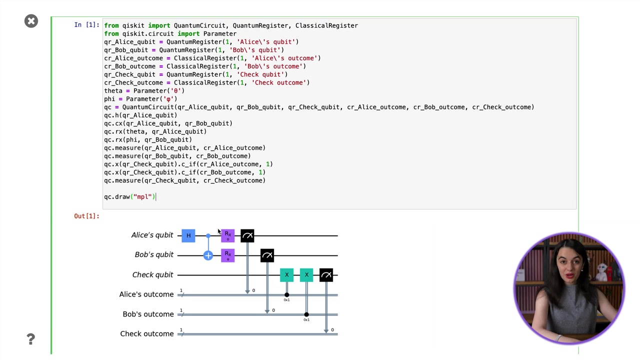 maximally entangled qubits is that whatever basis Alice and Bob choose to measure their qubits, if they choose to measure them in the same basis, their measurement outcomes will be correlated. For example, z-basis measurements will always give outcomes of zero-zero or one-one. 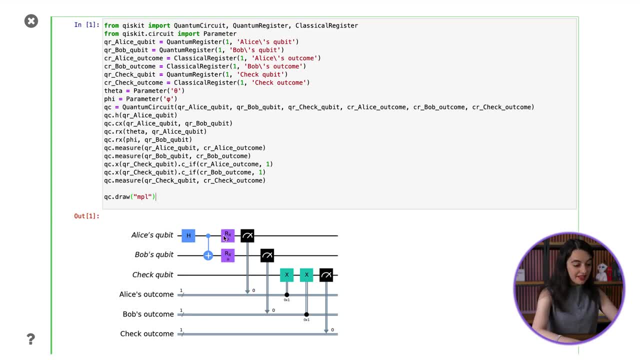 if both do x-basis measurements implemented by adding HadMod gates before the z-measurements, then again they'll always get outcomes of either 0, 0 or 1, 1, corresponding to measuring the two qubits to be in the plus-plus or minus-minus states respectively. 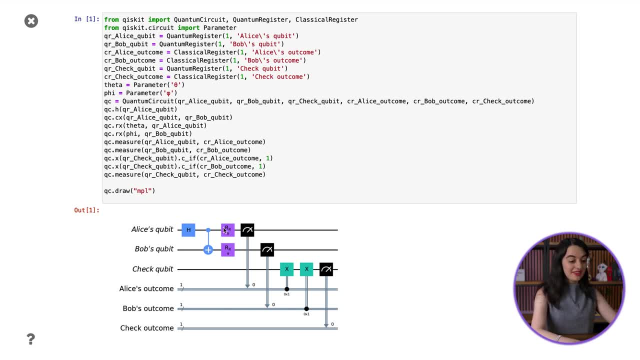 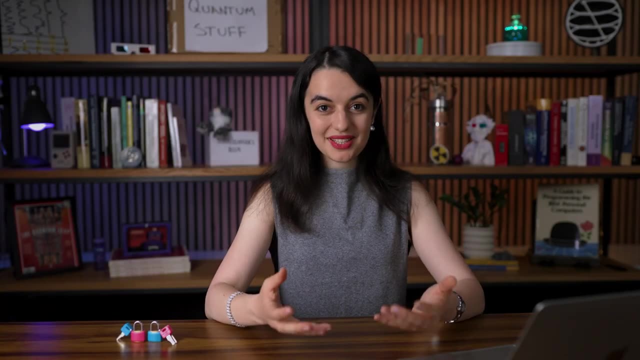 So, even though Alice and Bob are free to choose the bases in which they measure their qubits independently, somehow their measurement outcomes conspire to always be the same, making the check qubit always 0.. Now there are classical systems which have correlations in multiple properties. 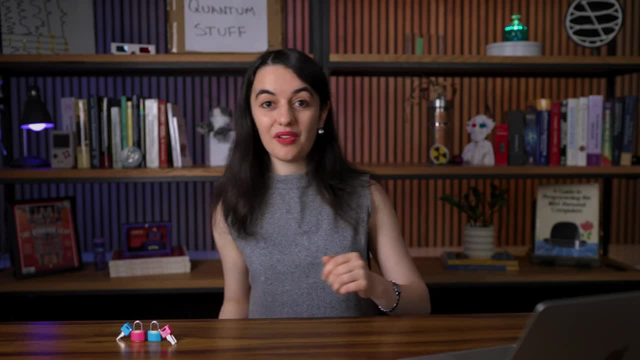 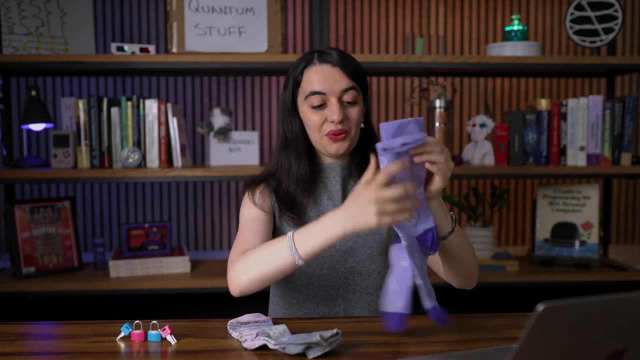 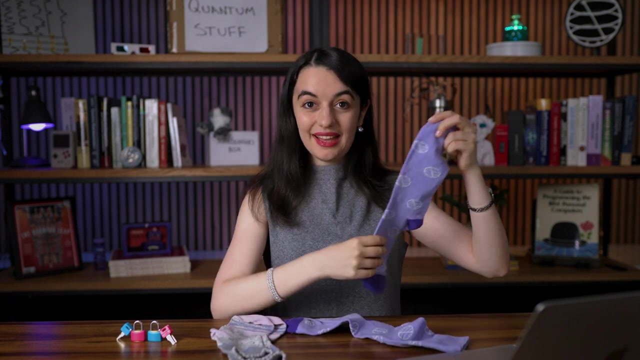 For example, consider Alice and Bob each having one of a pair of socks. The pair is either a large pair of kiss-kits socks or a small pair of stripy socks. Now, if Alice's sock has kiss-kit logos, then she knows that Bob's sock must also. 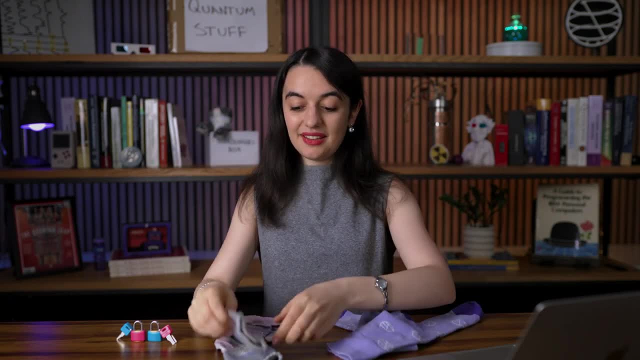 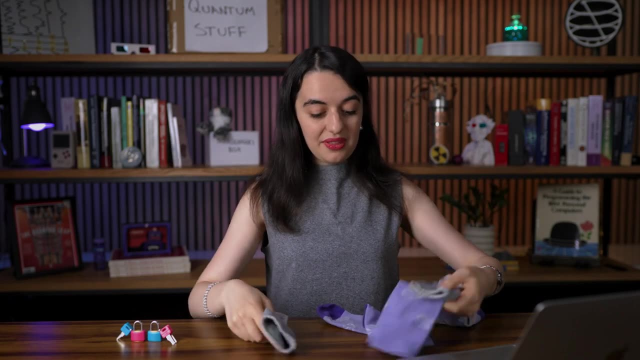 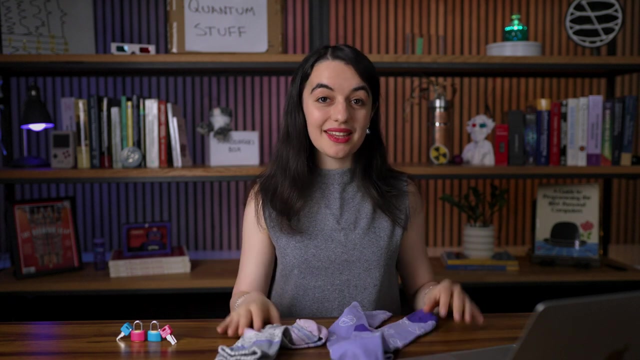 have kiss-kit logos, And if Alice's sock is small, then she knows that Bob's sock is also small. So both the size and the colour of the socks is fully correlated. Now the difference in the quantum case is that a qubit cannot have a definite state. 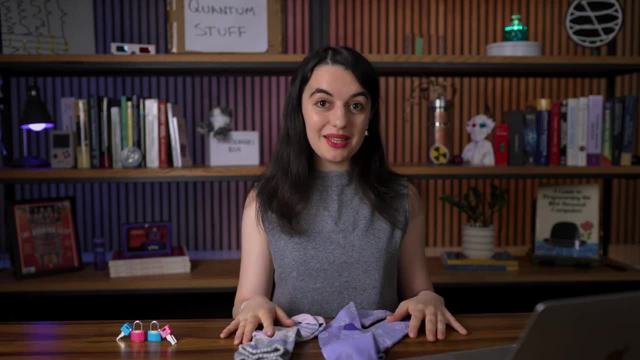 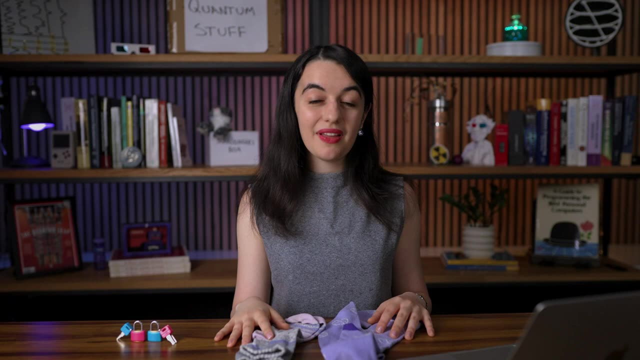 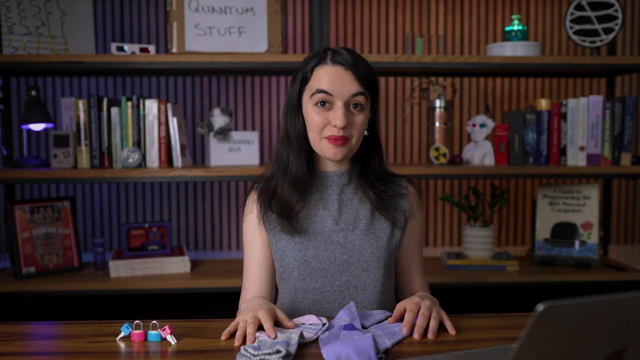 in the qubit, So you can see that the socks can't have a well-defined pattern and size simultaneously. This is a version of Heisenberg's uncertainty principle, which says that a particle can't simultaneously have a definite position and momentum. This property is what makes it strange for Alice and Bob's measurement outcomes to be fully correlated, in whatever basis they do their measurements. Using the sock analogy, it's like the socks can't have a well-defined pattern and size simultaneously. So it seems like Alice's choice of measurement basis has some instantaneous effect on Bob's qubit, since Bob's qubit seems to know what measurement outcome to give so that it will. 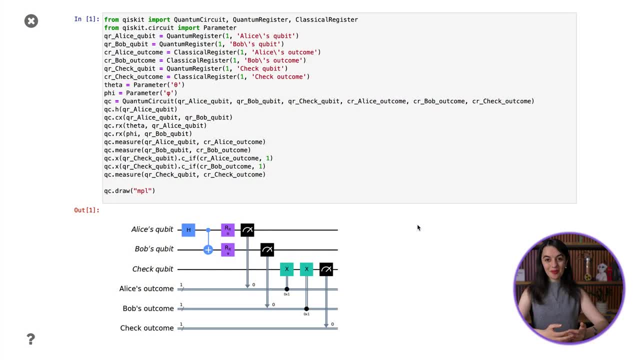 be correlated with Alice's. Bell's theorem is often quoted to support this viewpoint. Bell's theorem considers a class of local theories called hidden variable models. In terms of the quantum circuit, the condition of a local variable model is the same as the. 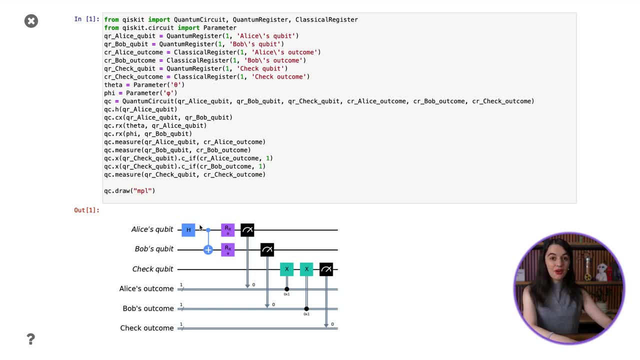 condition of a local variable model. In other words, the distribution of Alice's measurement outcomes is described by a variable which only depends on theta and not on phi, Whereas Bob's measurement outcomes can be described by a variable which only depends on phi and not on theta. 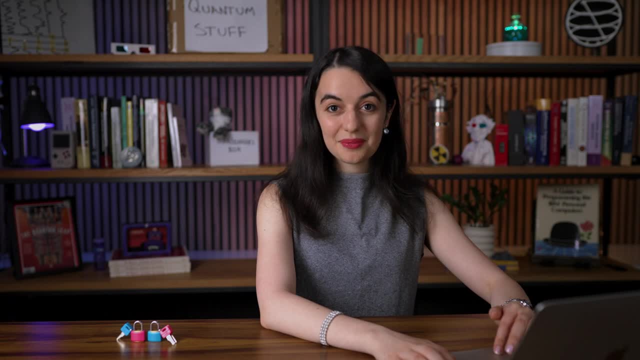 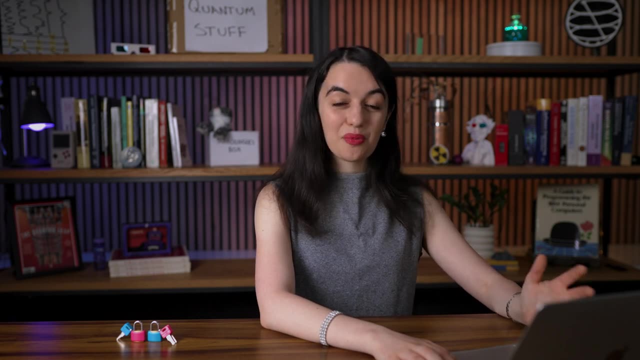 These assumptions place constraints on Alice and Bob's measurement outcomes, which are violated by quantum mechanics. This is why they are called hidden variable models. This is why they are called hidden variable models, But quantum mechanics cannot be described by a hidden variable model. 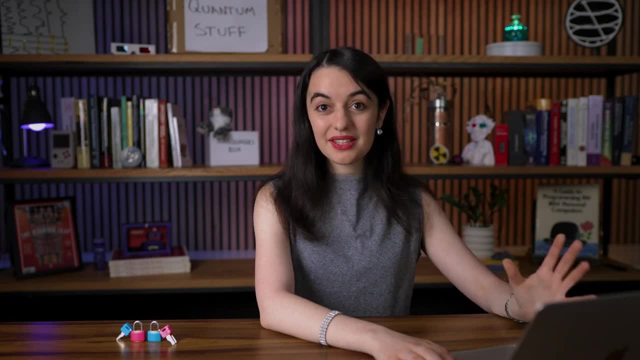 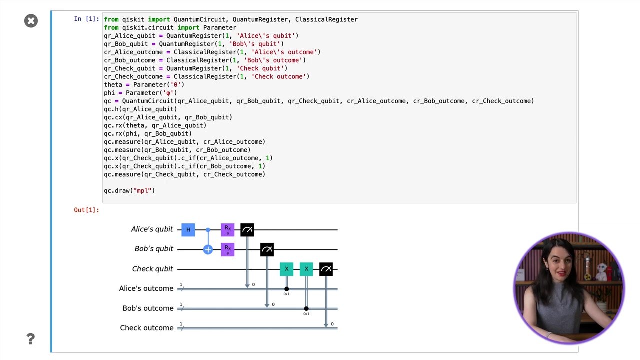 The type of locality ruled out by ruling out. this class of local theories is called Bell nonlocality. However, Bell's theorem only rules out one class of local models for quantum theory. To explain the alternative local formulation, we need to consider an alternative quantum. 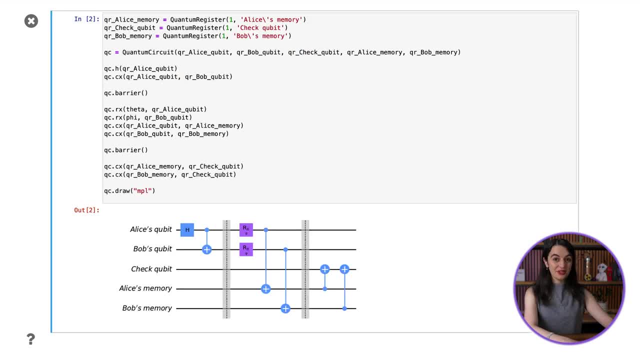 circuit. This is identical to the previous quantum circuit, Except that we change the classical registers of Alice and Bob's measurement outcomes to quantum registers. Then Alice and Bob's measurement operations become control-knot gates, such that if the control is 0, the memory will stay in the 0 state and if the control is 1, the memory. 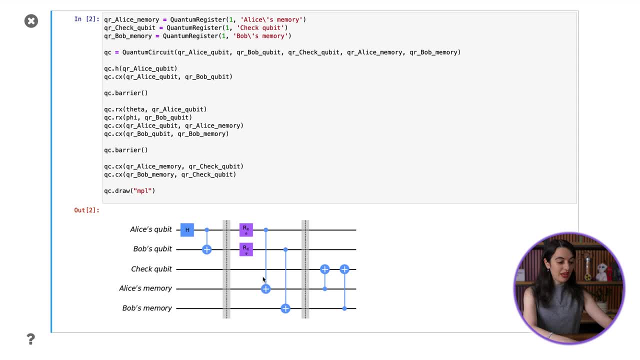 will be flipped to the 1 state so that each memory qubit stores the outcome of measuring one of the entangled qubits. As mentioned in previous videos, switching measurements for c-knot gates can be done with no difference to the final distribution of measurement outcomes, known as the principle. 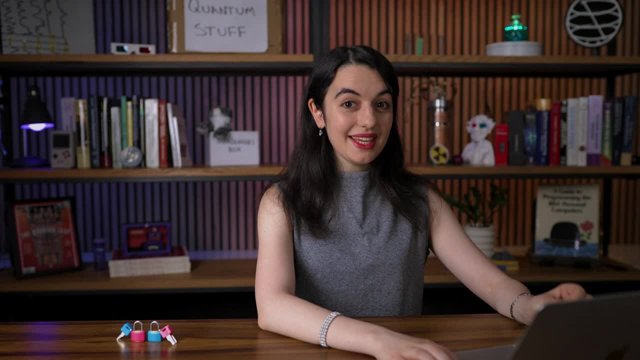 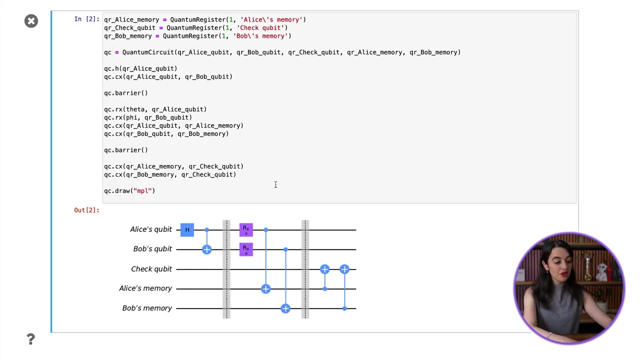 of deferred measurement in quantum computing. However, a key difference to the Bell-type approach is that here we do not assume that Alice and Bob have single probabilistic measurement outcomes. Our overall description of events here is unitary, maintaining the overall entangled superposition of the multiple measurement outcomes that happen after the simple distribution. This can be observed in the following diagram, with the exact same equation In the above diagram, Alice and Bob have single probability measurement outcomes. Here Alice and Bob have one conditional probability measurement outcome, while other algorithms 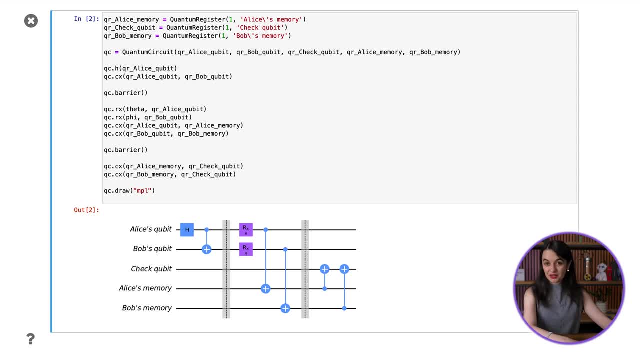 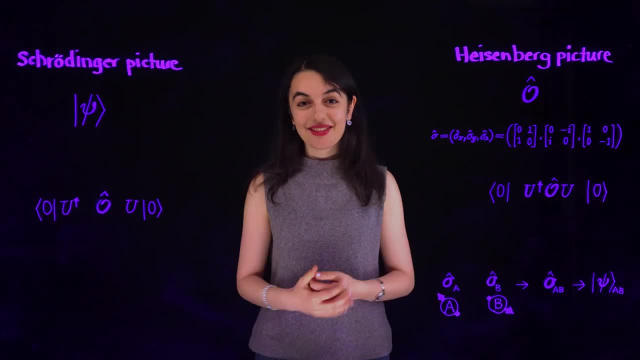 that Alice and Bob could retrieve, freeing it from the assumptions of Bell's theorem. Now, to understand this approach, let's go to the lightboard. To understand the local account of the EPR-Ford experiment, we need to shift from our usual 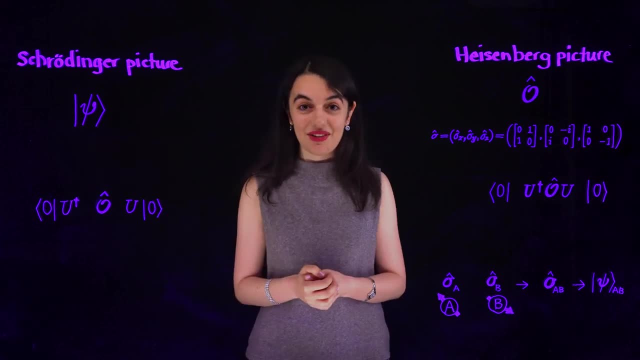 description of quantum mechanics using state vectors, which is known as the Schrödinger picture, to describing it in terms of observables, known as the Heisenberg picture. These two pictures are mathematically equivalent in the sense that they lead to exactly the same. 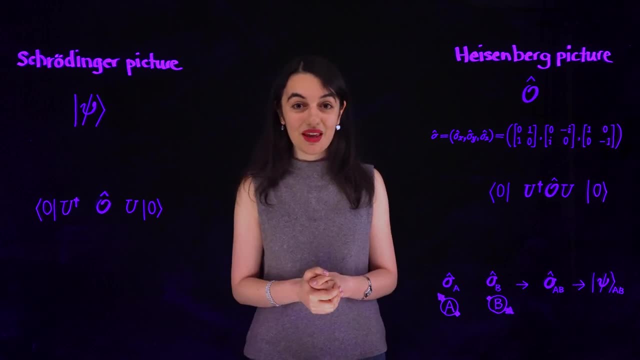 predictions about our measurement outcomes in quantum mechanics. but only the Heisenberg picture makes the local account of quantum mechanics explicit. To understand the difference between state vectors and observables, let's consider taking the expectation value of some observable when we have evolved a quantum system starting. 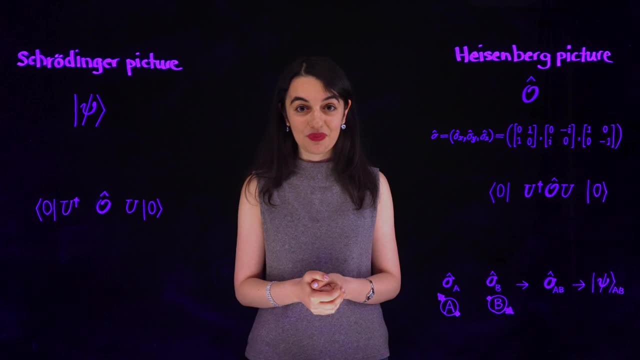 in the state zero by some unitary gate u. The observable could, for example, be the Pauli x, y or z observables. if we wanted to find out the average outcome of making x, y or z measurements respectively, 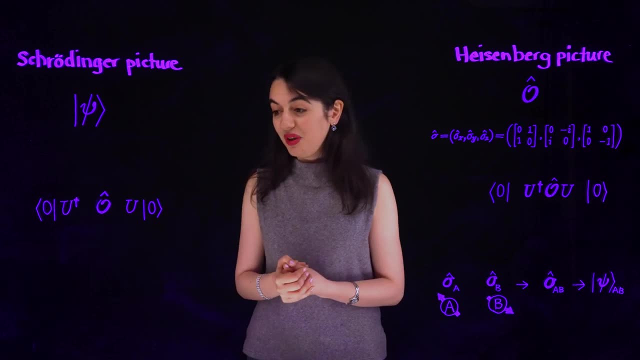 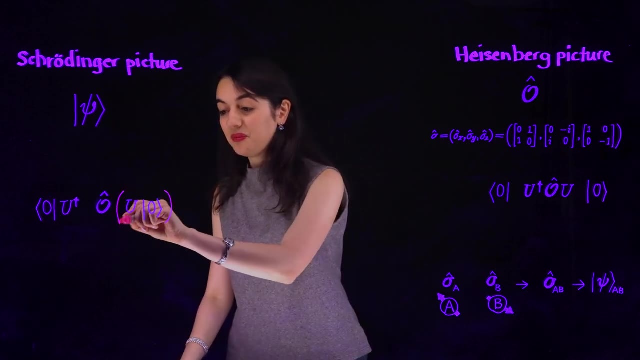 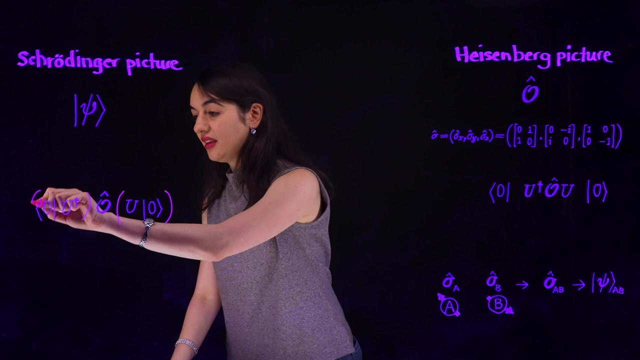 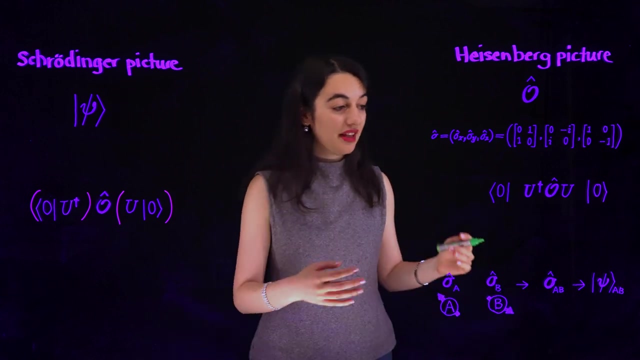 To work out the expectation value. in the Schrödinger picture, we first evolve the initial state from zero using the unitary gate u, and then we sandwich our operator for the observable in between the bra and ket. Now, in the Heisenberg picture, we instead first evolve our observable using the unitary 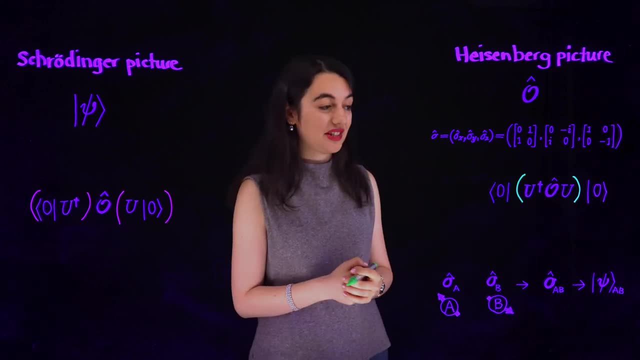 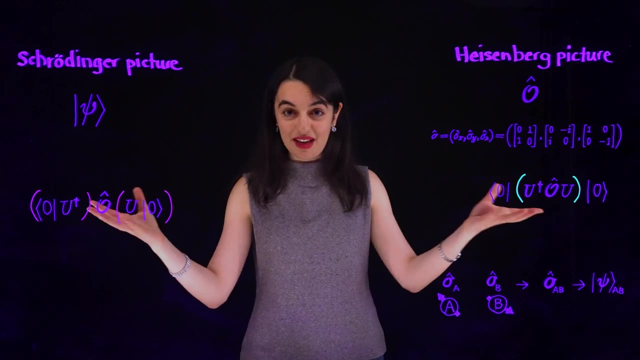 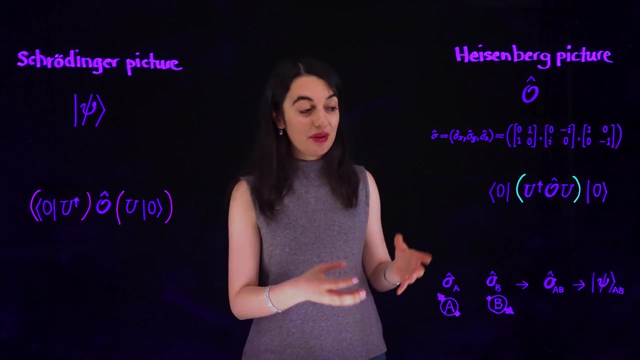 gate u, and then we sandwich it in between the initial state vector. You can see that the final two expressions we get for the expectation value are exactly the same. Now, the properties of an individual quantum system can be fully described by evolving its observables. 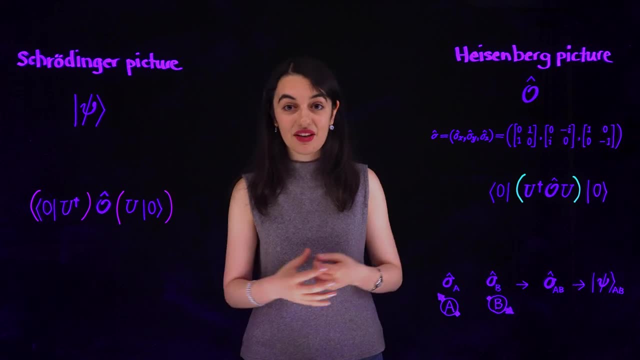 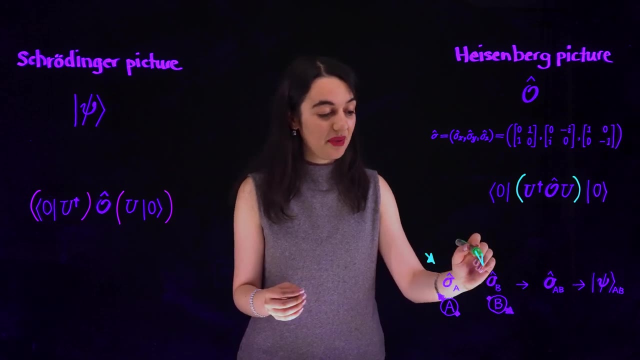 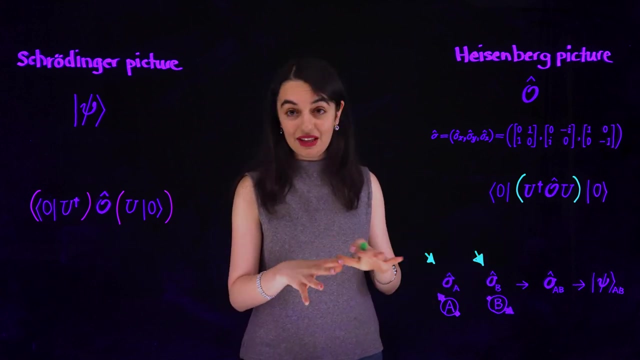 The observables give us local and complete information about quantum systems, in the sense that if we have some system A and another system B, then if we know their individual observables, then we can work out the joint observable of A and B and from that we could. 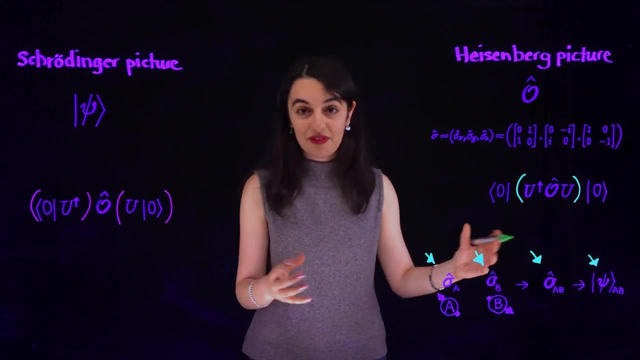 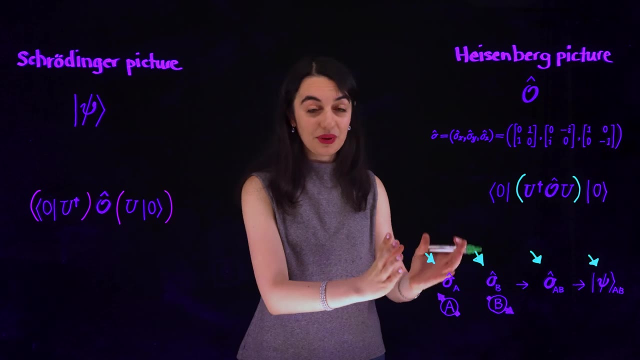 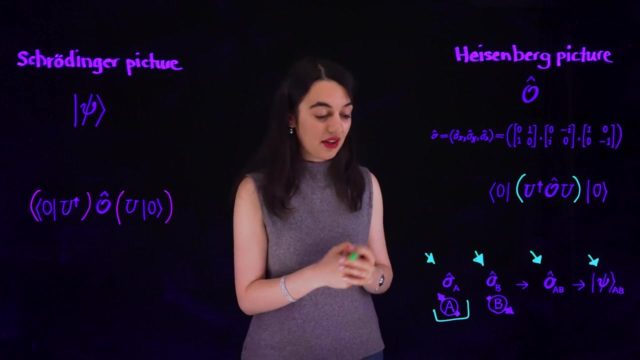 work out the global state vector, Even if A and B are entangled. Now, applying a quantum operation to one quantum system can only affect the observables of that quantum system. It can't affect the observables of another system when they don't directly interact. 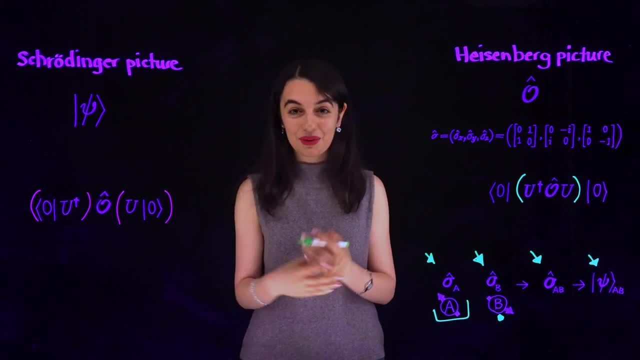 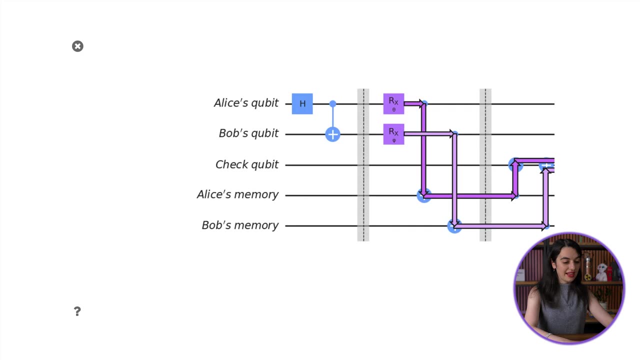 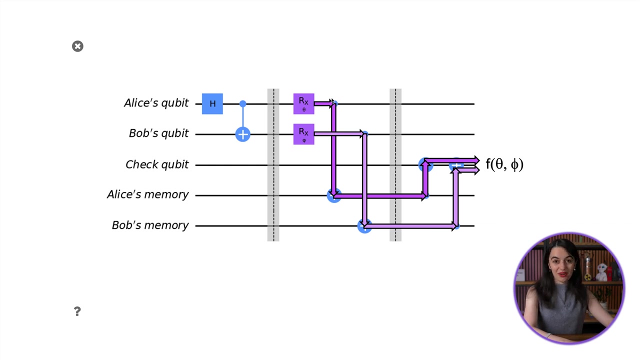 Let's see how this helps us resolve the EPL thought experiment in our quantum circuit. 1. With the local flow of information in this quantum circuit. I have added some arrows So we can see here that there is a direct quantum operation from Alice's qubit to Alice's. 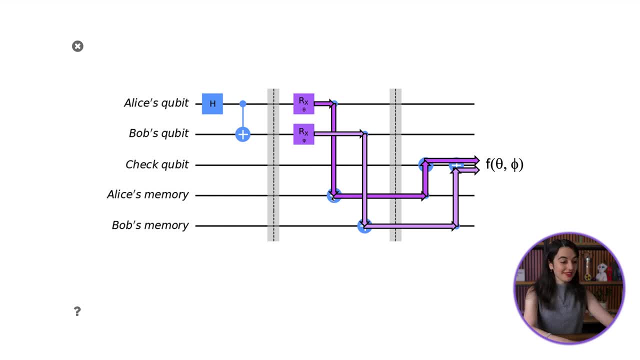 memory, meaning that the observables describing Alice's memory qubit can depend on the parameter theta. Similarly, the observables describing Bob's memory qubit can depend on the parameter phi 2.. Next we have the two CNOT gates that implement the parity check with the check qubit. 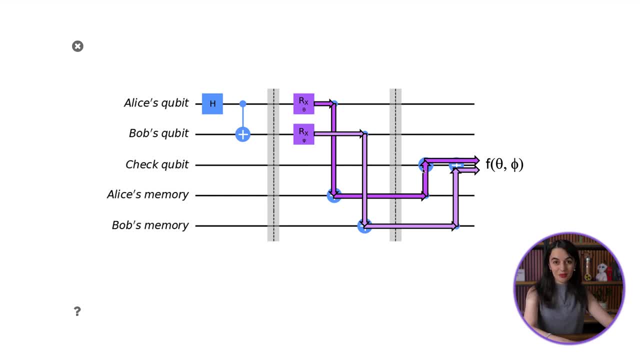 One of them acts directly between Alice's memory and the check qubit, so that the check qubit's observables can depend on theta, and the other acts directly between Bob's memory and the check qubit, so the check qubit's observables can also depend on phi. 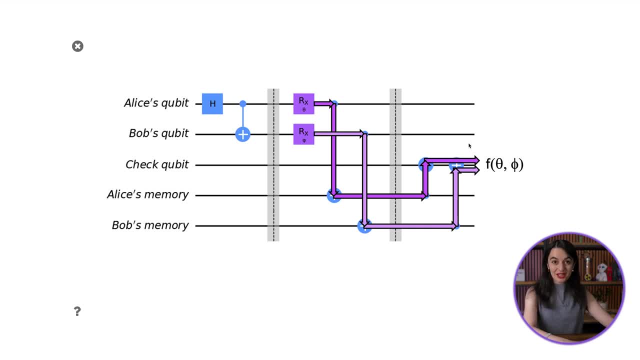 Therefore, the final outcome of the check qubit, which reveals whether or not Alice and Bob's qubits are correlated, can depend on theta 3.. We can explain this dependence in a fully local way, tracking the flow of information about which bases Alice and Bob chose to measure their qubits all the way through the circuit. 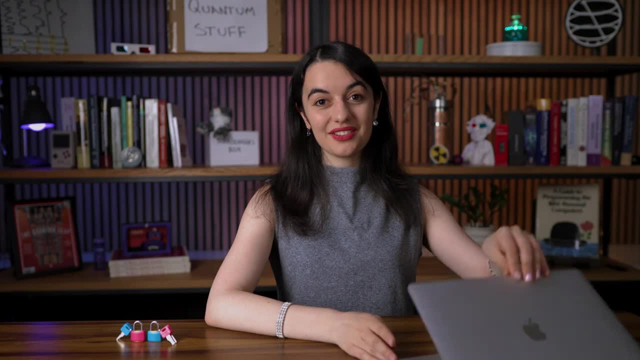 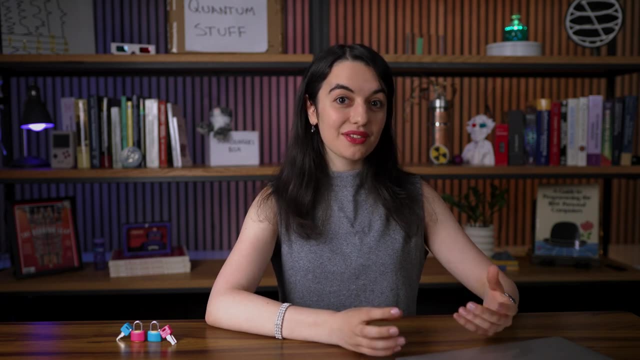 step by step. 4. The fully local formulation of quantum theory is not just a neat way to track the flow of quantum information. It is also important for the broad goal of recognizing the flow of quantum information. 5. We have the broad goal of reconciling quantum theory with gravity, which is one of the biggest. 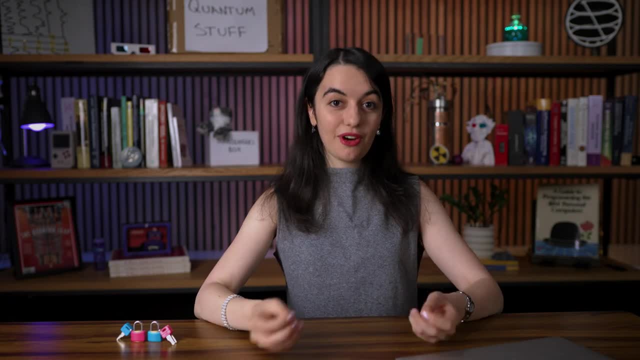 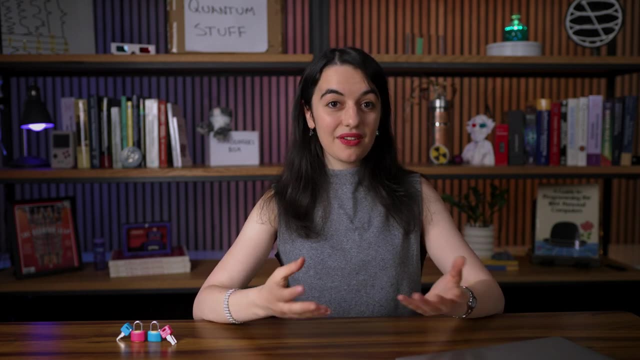 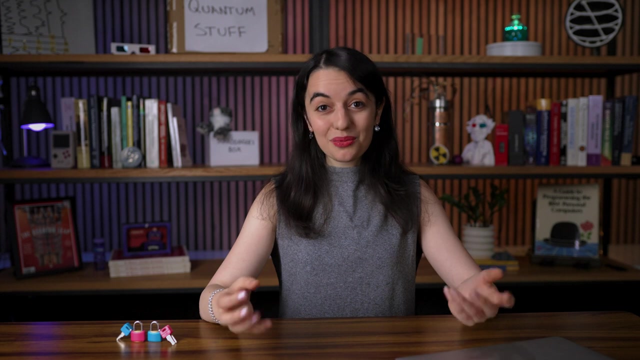 problems in fundamental physics. Our best theory of gravity is given by general relativity, which is local in the sense that Einstein described. We don't yet have a good theory that combines quantum mechanics with general relativity, but having a local formulation of quantum theory is one important step towards finding 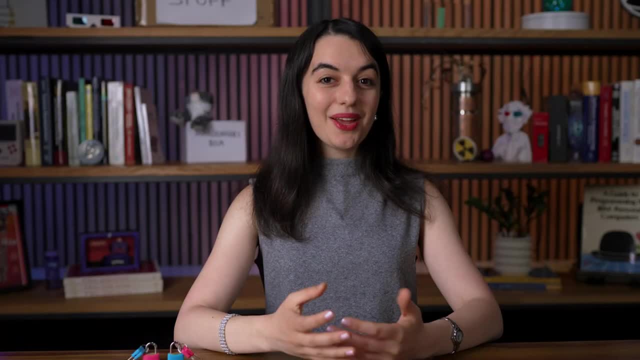 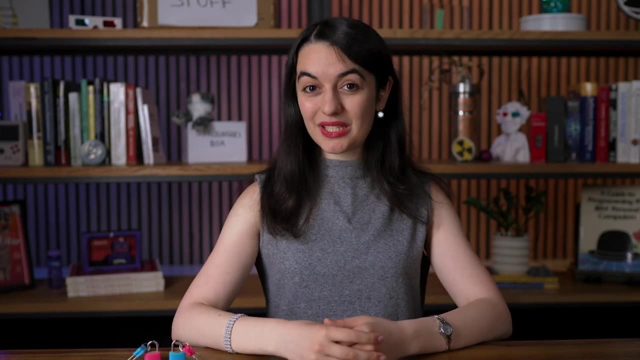 a way to reconcile the two theories. 6. Now, even though quantum entanglement can be explained without needing spooky action at a distance, it still has strange consequences. We can imagine this by representing Alice and Bob's entangled qubits by these colored 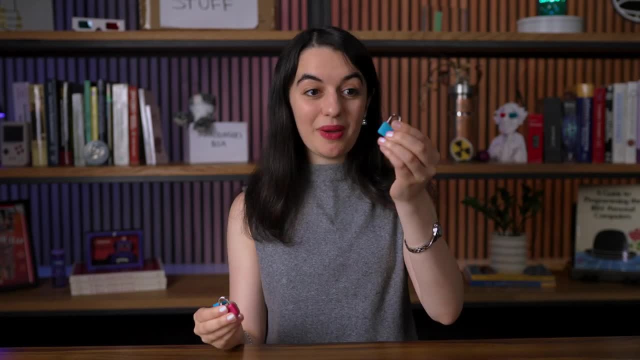 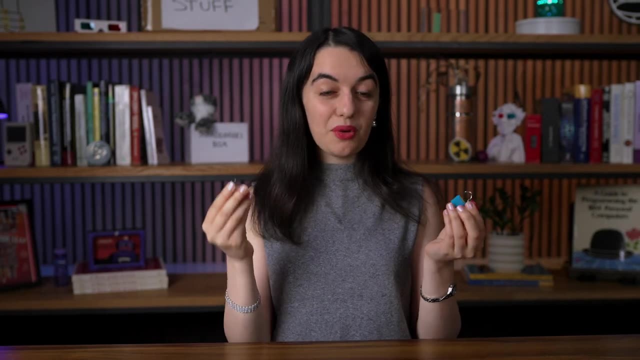 padlocks and keys. Let's say Alice has the blue padlock with the pink key and Bob has the pink padlock with the blue key. Now, when Alice and Bob's qubits are fully entangled, the value of the parameter theta is localized on Alice's qubit. 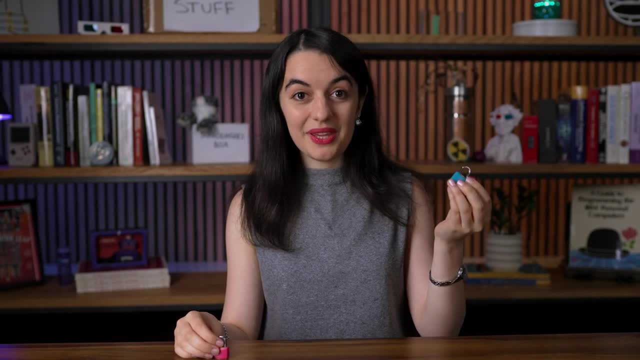 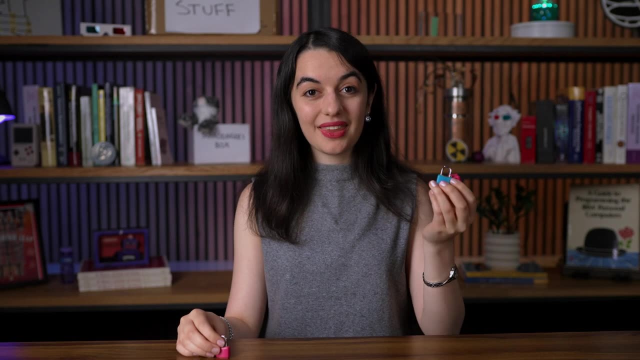 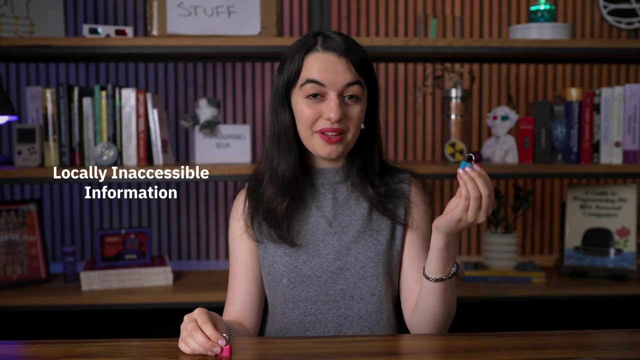 7. However, theta cannot be accessed by measurements on Alice's qubit alone, even if we had infinite copies of Alice's qubit. The value of theta is therefore locked up in Alice's qubit. This is called locally inaccessible information. 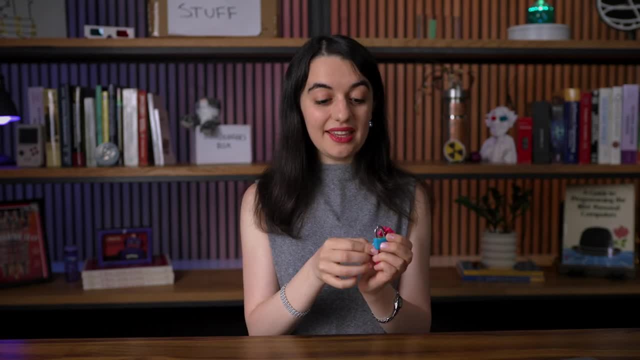 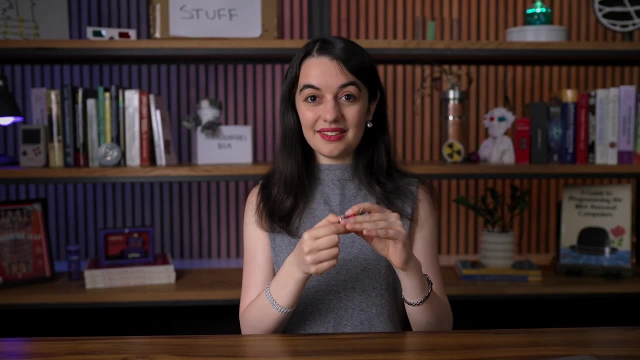 8.. Then Bob's entangled qubit acts as a key to unlock the information in Alice's entangled qubit 9.. Similarly, Alice's qubit acts as a key to unlock Alice's entangled qubit 10.. 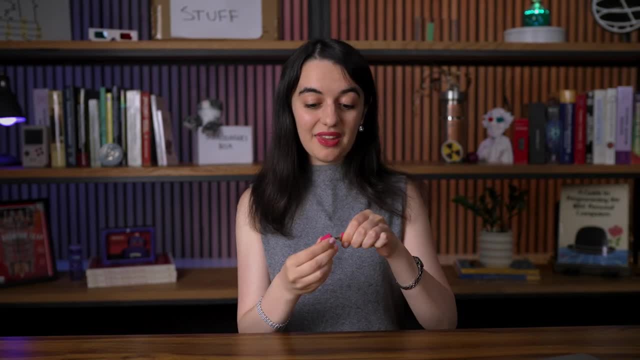 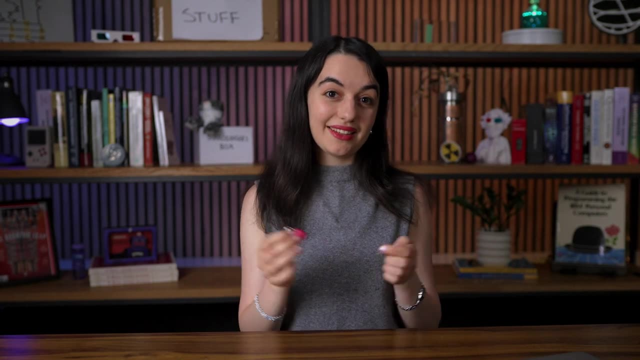 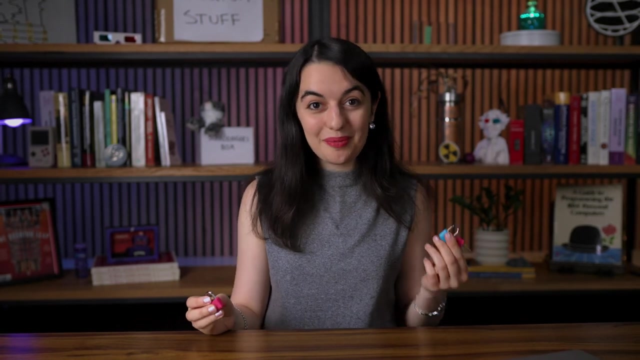 The value of theta acts as a key to unlock the information about the parameter phi that's stored in Bob's qubit 11.. Now the cool thing about locally inaccessible information is that, since it's not retrievable by measurements, it also can't be destroyed by measurements. 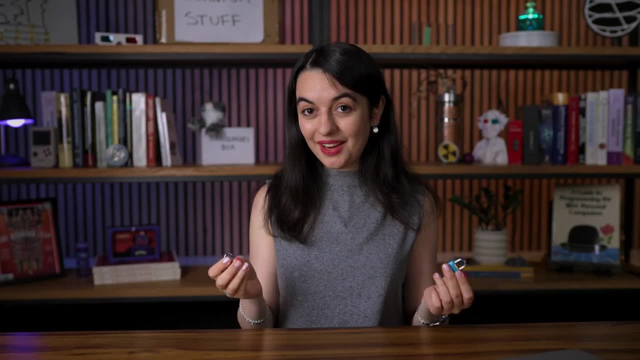 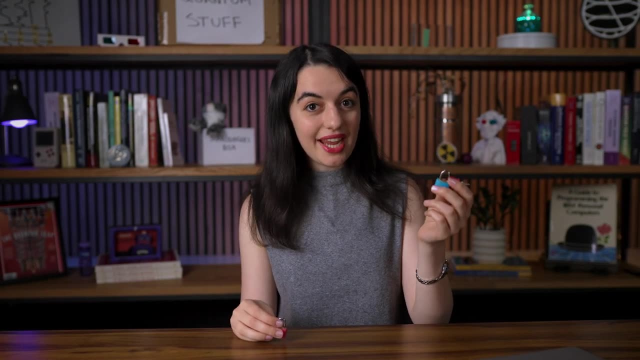 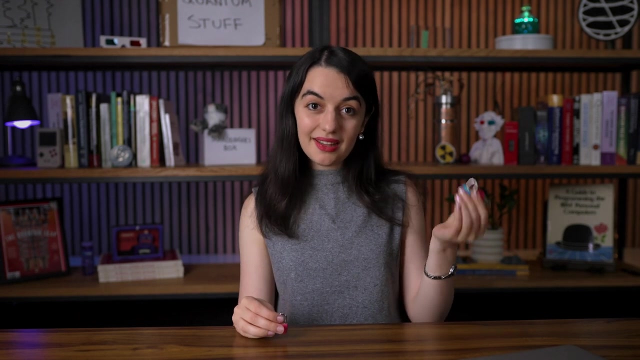 So this information is robust to decoherence. Alice's qubit can be measured in the z-basis again and again, and again and still retain the locked-up information about theta, which is why we can describe her measurements perfectly well using classical registers in our original quantum circuit. This robustness to decoherence, 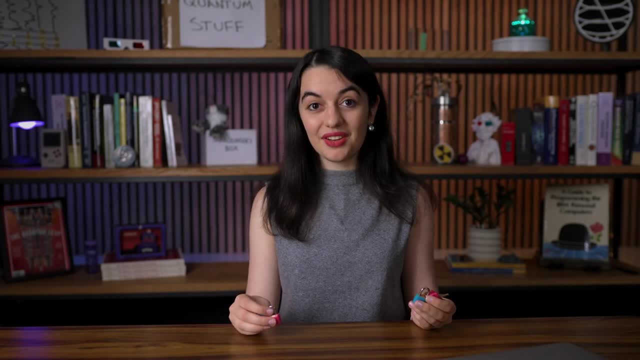 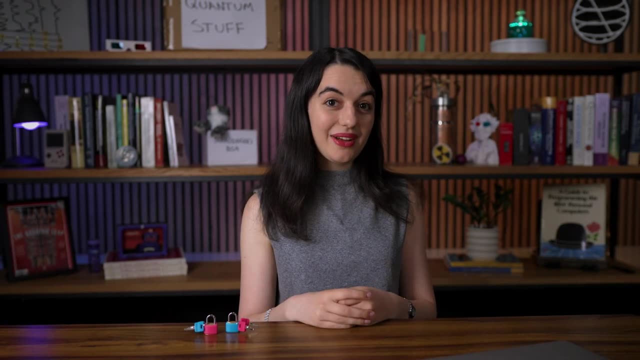 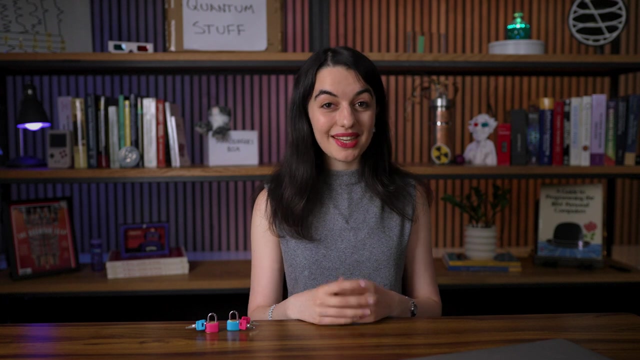 turns out to be the key to understanding how information really gets from one place to another in the quantum teleportation protocol. In the next video, I'll explain how we can implement quantum teleportation on a quantum computer and resolve the apparent paradox of using entanglement.